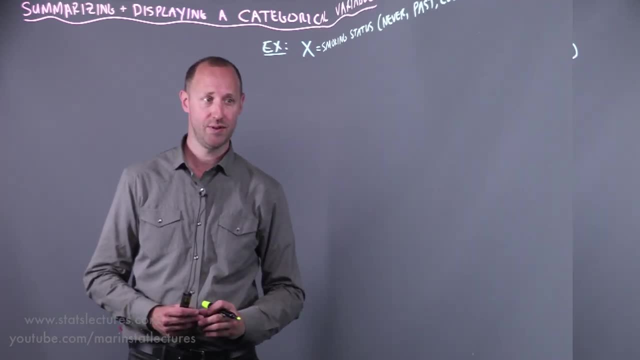 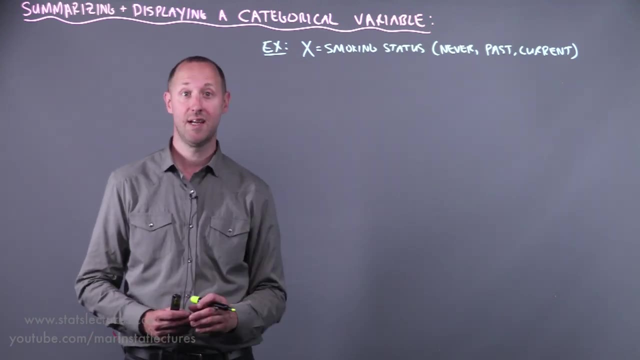 smoker, and we'll assume we've taken a sample size of 200. So here we like to use a simple example just for the sake of discussion. So the most relevant way to summarize a categorical variable is to count how many people fall into each of the categories or levels of the. 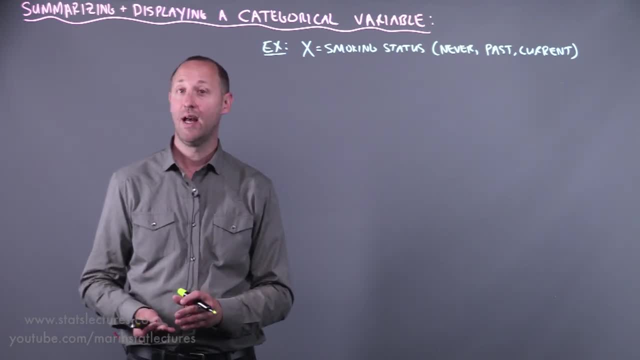 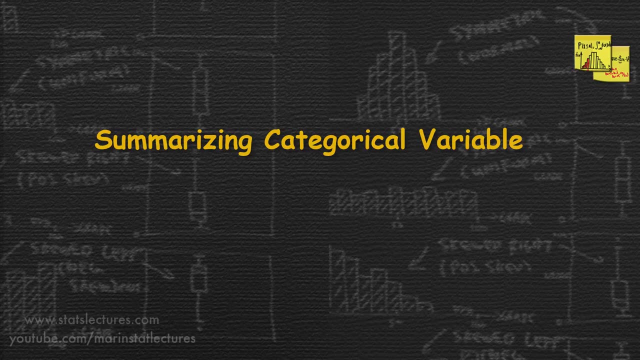 variable and then summarize that either using a frequency, a relative frequency, which also gets called a proportion, or a percentage. So let's take a look at doing that. The first thing we need to do is start by talking about a frequency table, or what sometimes gets. 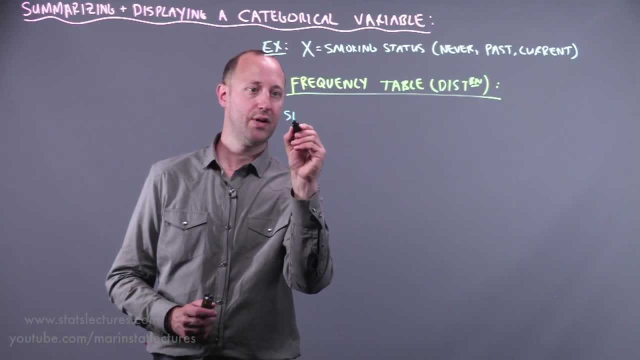 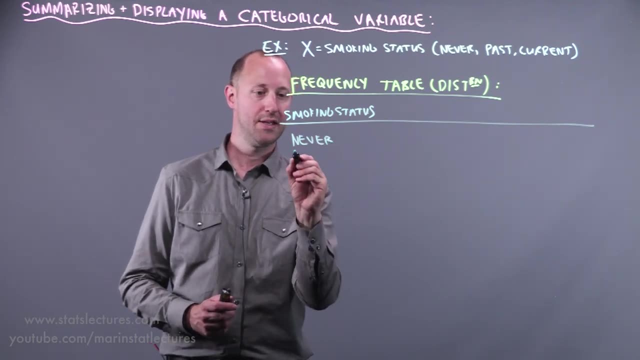 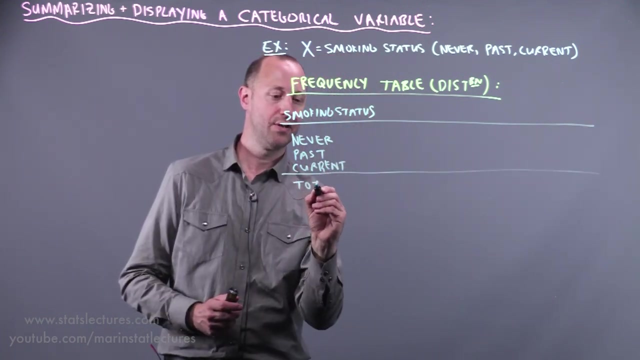 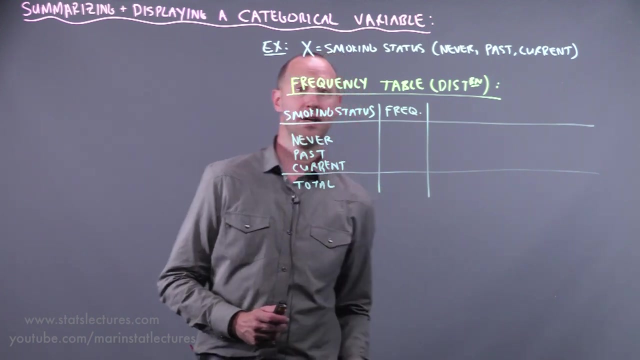 called a frequency distribution. So we have the smoking status And that again we've recorded as never, as past or current, And again here I'll put down the total. So here we can think of recording the frequency or the number that fall into each of these. 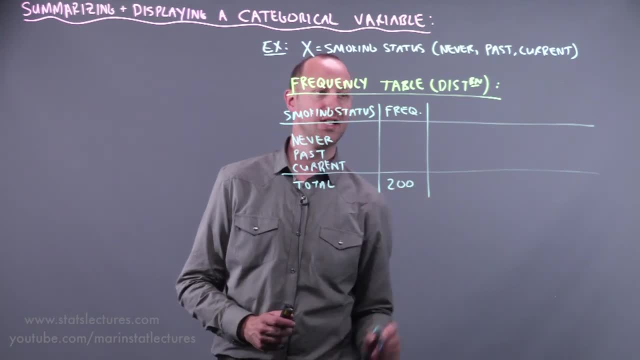 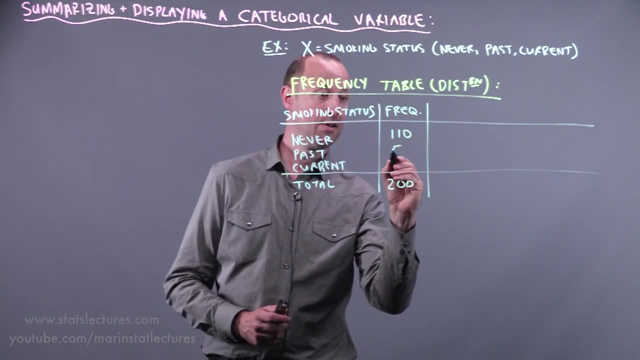 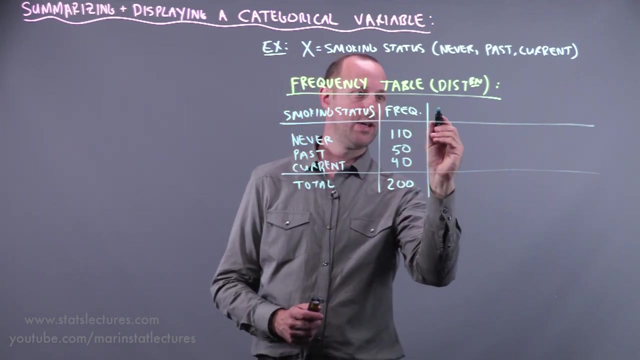 groupings for the categorical variable. So we've got a sample size of 200, and let's suppose that 110 responded as never smokers, 50 as past and 40 as current. Then, rather than recording the frequencies, we can convert this into a proportion, or what also gets reported as: 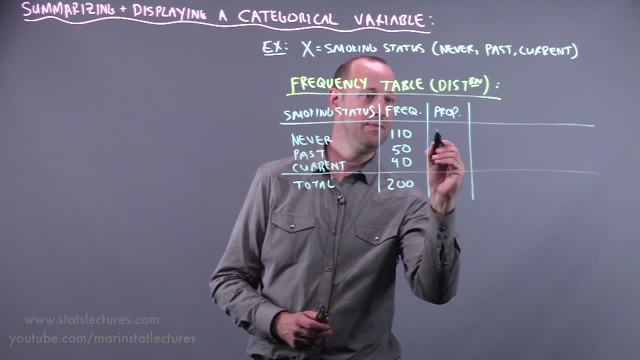 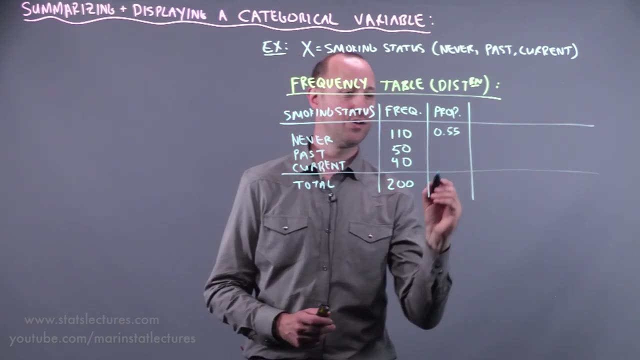 a relative frequency sometimes. So the 110 out of the 200 is 0.55.. The 50 out of the 200 is 0.25.. And the 40 out of the 200 is 0.55.. So this is the long term frequency. And next we've got a percentage ratio. So let's think about how we're going to calculate the percentage ratio of a smoke. So we've got, right at the top, the product ratio of a smoke. The quantity ratio of the smoke is the number that falls into each of the categories and 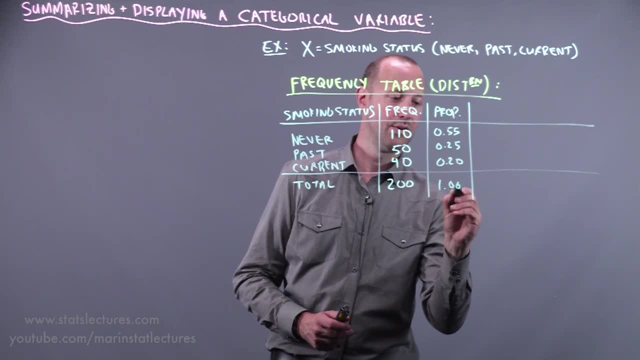 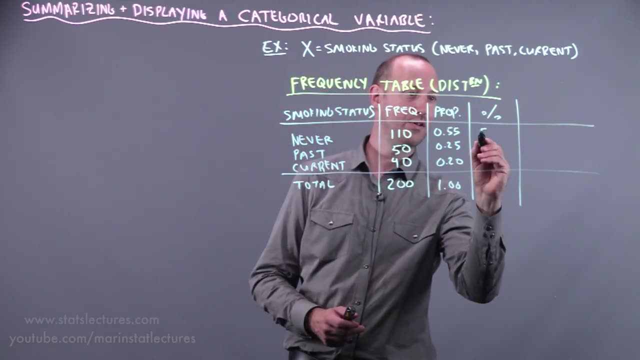 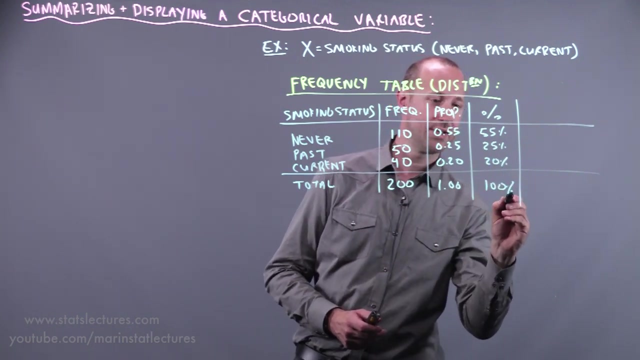 of the 200 is 0.20 for a total of 1.0, or we can also report these as percentages: 55 percent, 25 and 20 percent out of the total 100 percent. okay, so for the most part, a proportion or percentage. 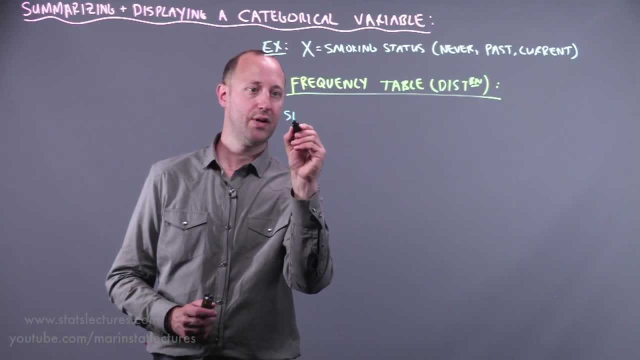 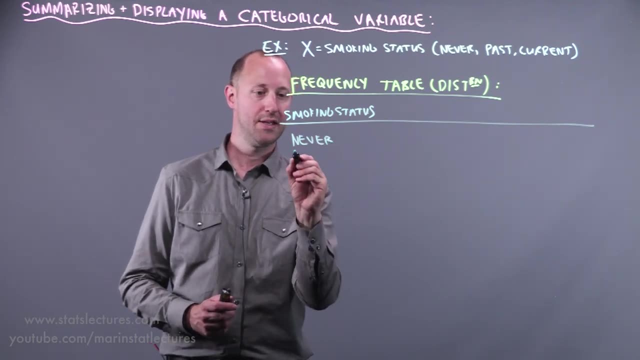 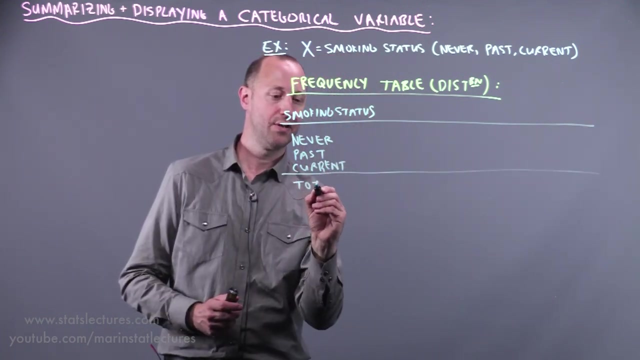 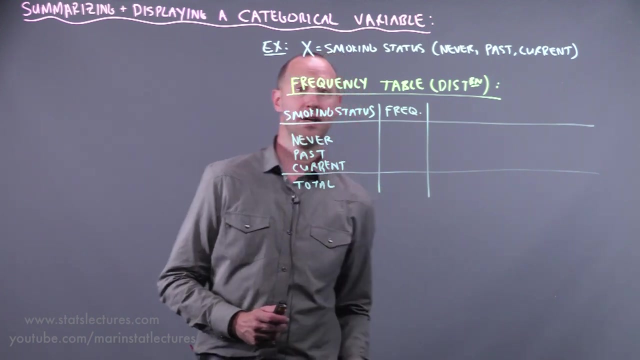 called a frequency distribution. So we have the smoking status And that again we've recorded as never, as past or current, And again here I'll put down the total. So here we can think of recording the frequency or the number that fall into each of these. 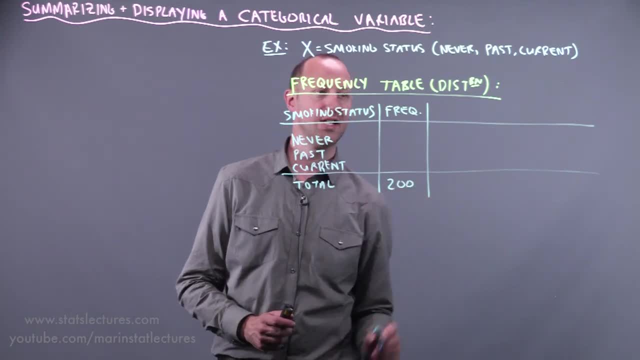 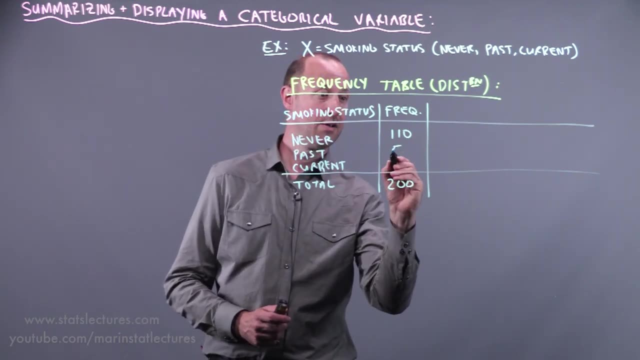 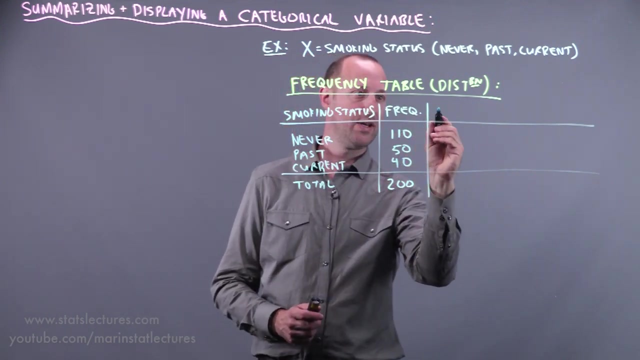 groupings for the categorical variable. So we've got a sample size of 200, and let's suppose that 110 responded as never smokers, 50 as past and 40 as current. Then, rather than recording the frequencies, we can convert this into proportion, or it also gets reported as a relative. 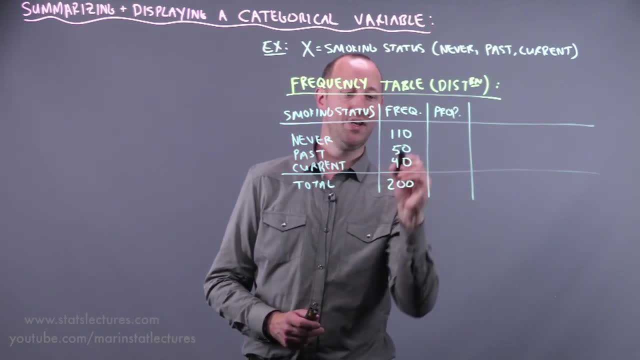 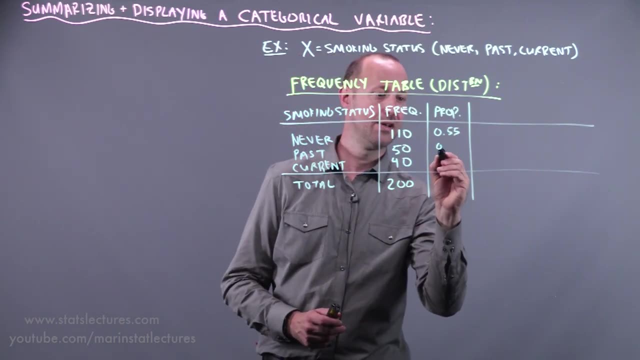 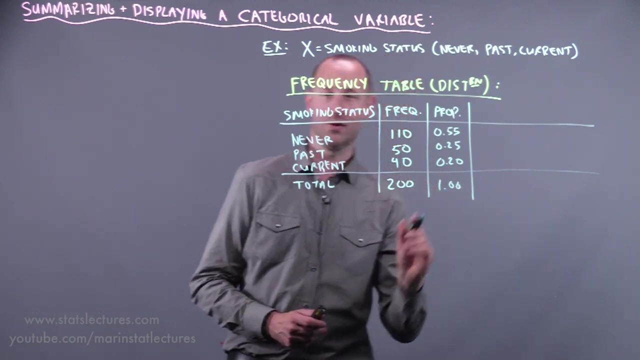 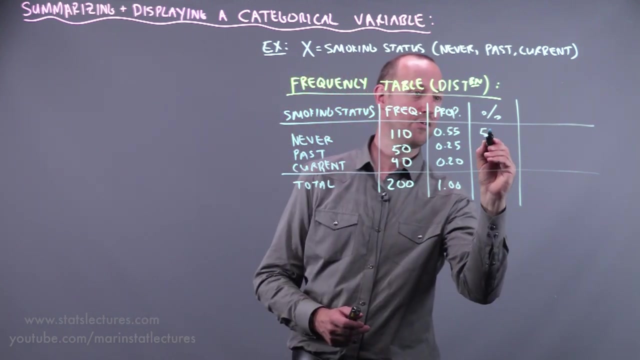 frequency sometimes. So the 110 out of the 200 is 0.55.. The 50 out of the 200 is 0.25. And the 40 out of the 700 is 0.. săf rápido of the 200 is 0.20, for a total of 1.0. or we can also report these as percentages: 55 percent, 25. 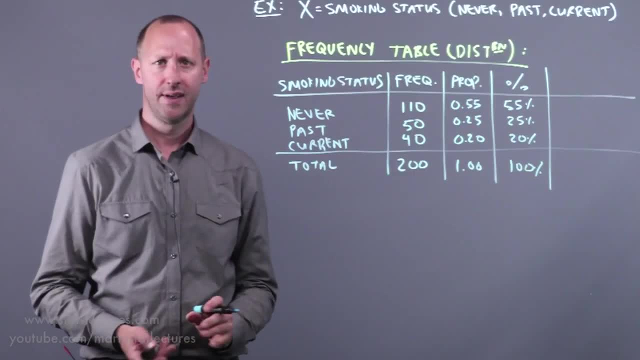 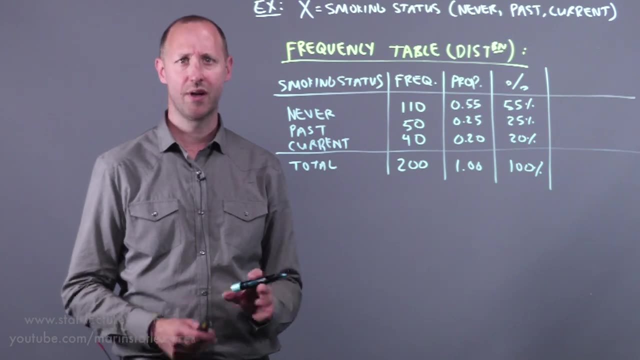 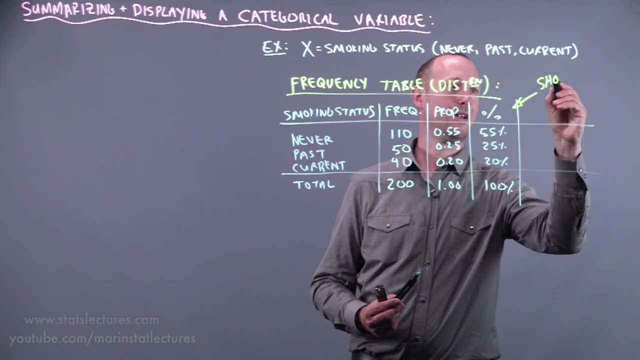 and 20 percent out of the total 100. okay, so for the most part, a proportion or percentage. while there are slight technical differences, we'll use the two for the most part interchangeably when we talk about things now. an important note about these is that this table here again shows the 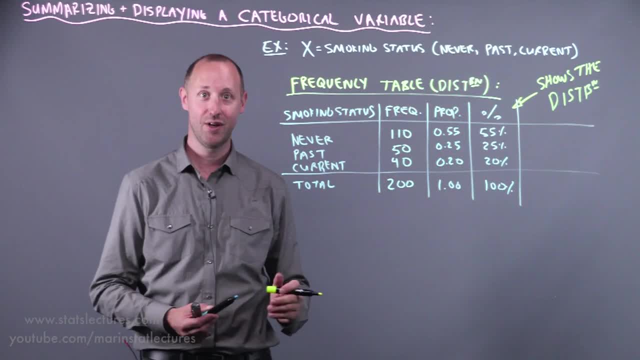 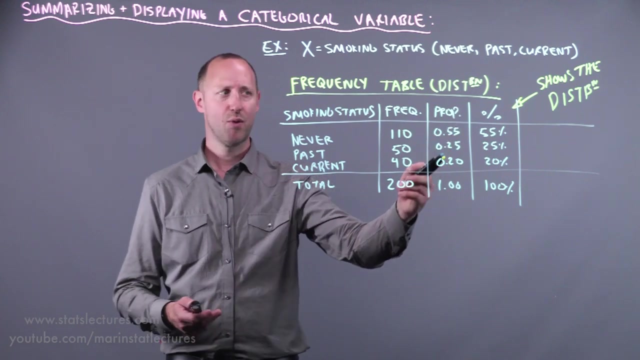 distribution. again, that's a keyword: statistics- you're going to hear that word thrown around a lot. how are cases or individuals distributed amongst the different levels or categories of this categorical variable? so a suggestion: when you have larger sample sizes, it's often a bit more meaningful to report the proportion or the percentage falling in each category. 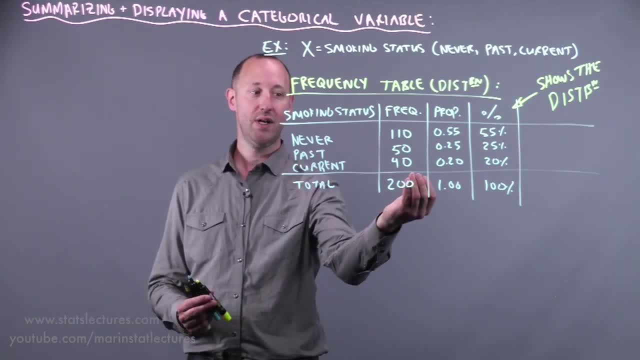 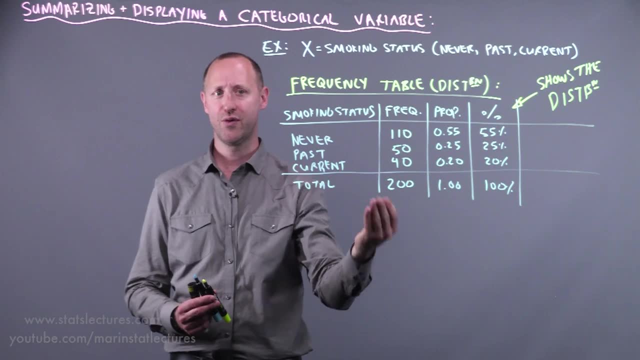 if you had smaller sample sizes. suppose we only had 20 individuals and we had 11 falling as never smokers. five is past and four is current. reporting those frequencies is going to be a bit more meaningful or easier to interpret, rather than reporting the percentages or proportions which can. 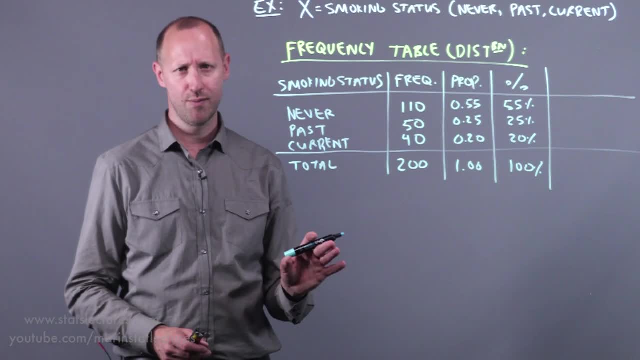 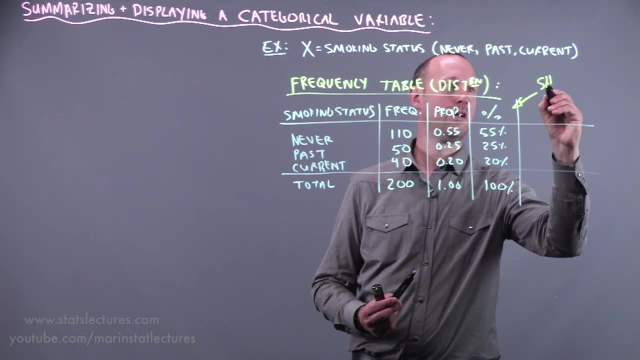 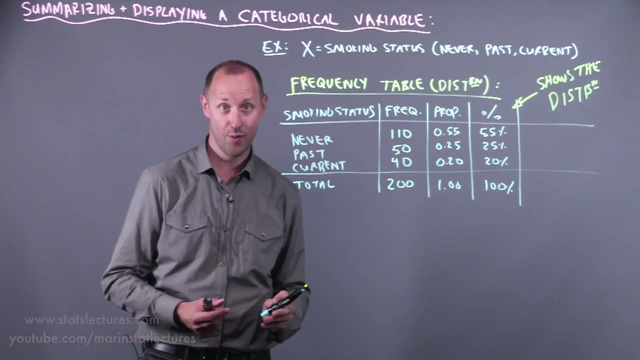 while there are slight technical differences, we'll use the two for the most part interchangeably when we talk about things now. an important note about these is that this table here again shows the distribution. again, that's a keyword: statistics- you're going to hear that word thrown around a lot. how are cases or individuals distributed amongst the different? 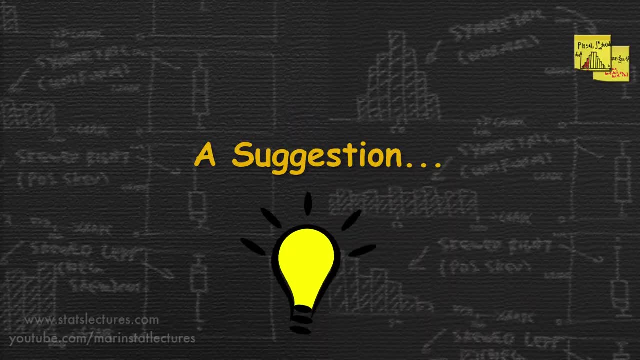 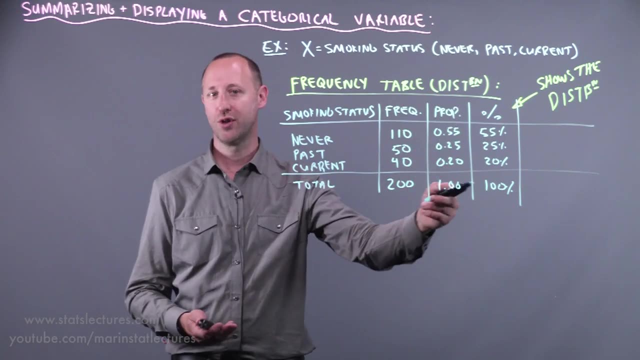 levels or categories of this categorical variable. so, on a suggestion, when you have larger sample sizes, it's often a bit more meaningful to report the proportion or the percentage falling in each category of the sample. so we're going to go ahead and do that, and we're going to go ahead and do. 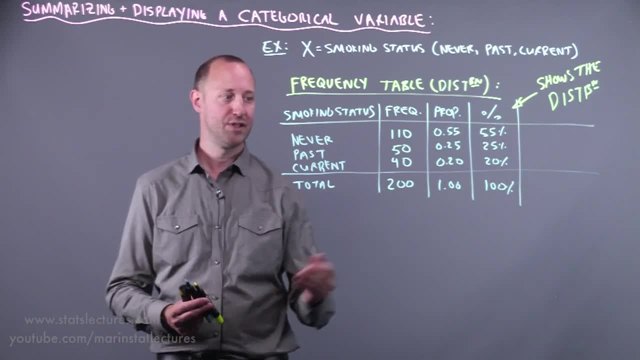 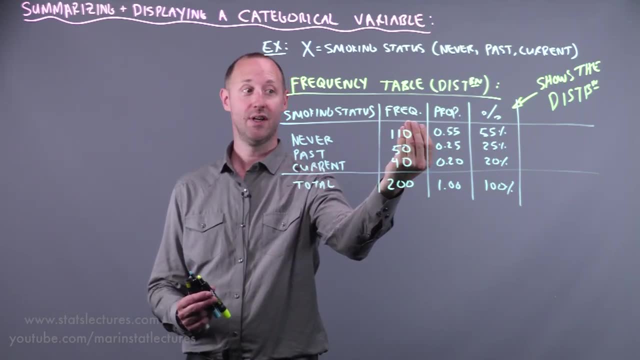 the same thing with the smaller category. if you had smaller sample sizes, suppose we only had 20 individuals and we had 11 falling as never smokers. 5 is past and 4 is current. reporting those frequencies is going to be a bit more meaningful or easier to interpret, rather than reporting the 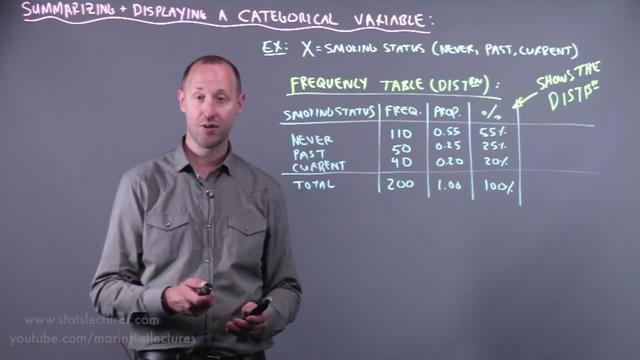 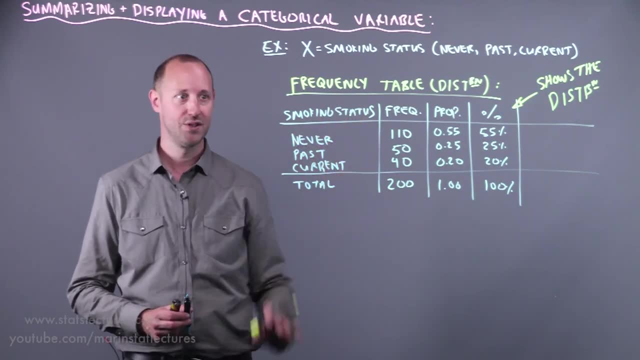 percentages or proportions, which can be a bit misleading with smaller sample sizes. now, if we want to make a plot of these, right, it's nice if we can make a visual of this table rather than just looking at a table of numbers, especially when we have lots of categories. 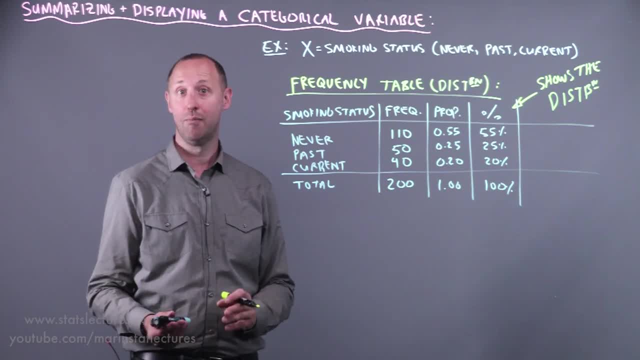 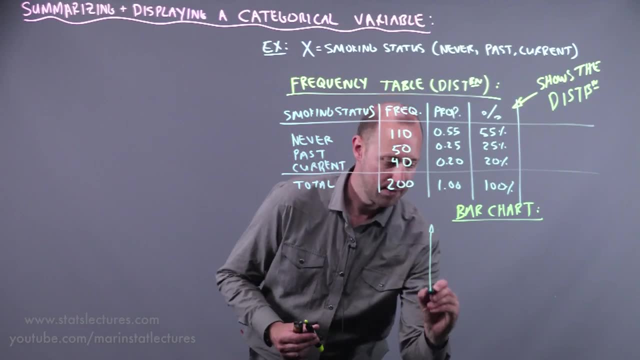 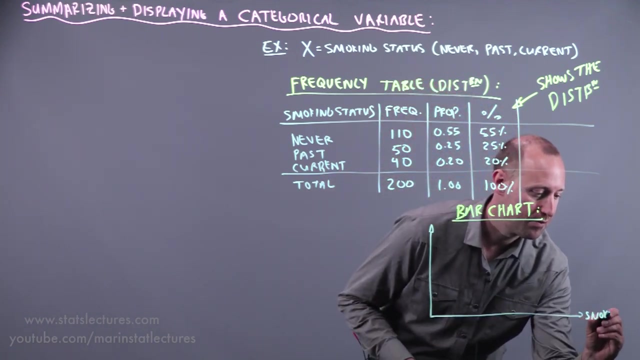 or the table gets bigger. we can make either a bar chart or a pie chart. so first let's start by talking about the bar chart. a bar chart has along the x-axis the variable. so here we're looking at smoking status again. this was recorded as never. 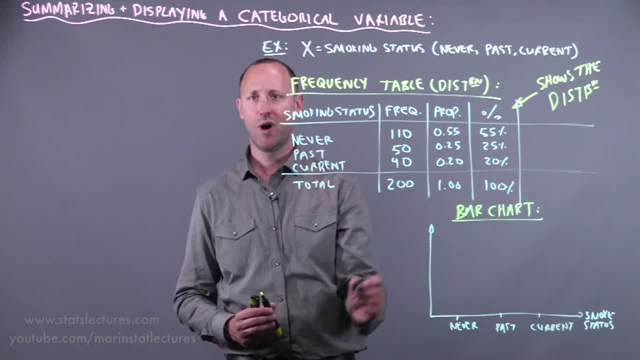 past or current, and along the y-axis we can put the frequency, the proportion or the percentage right. so when we were once filmed, we focused on two methods. we were trying time: text, the sample, one psychological nature. each promise 0.1, the probability ratio: 1.1, about 1.1 if we were 10 points. 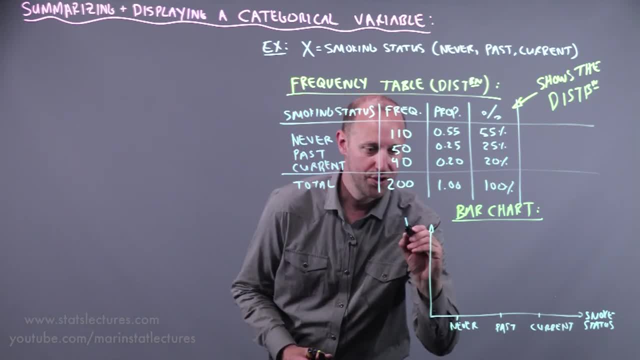 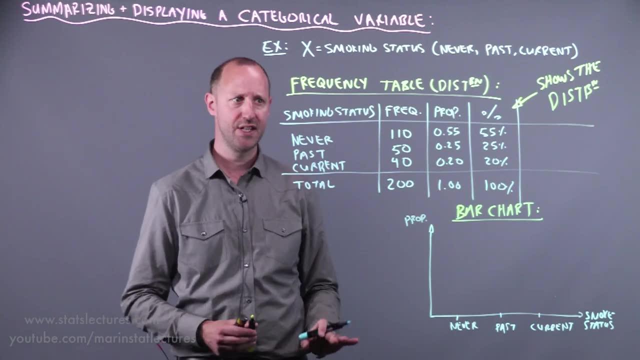 The plot's gonna look the same. I'm gonna choose to put the proportion here, Since our sample size is not very small. I think it's more meaningful to report proportions or percentages, and I'll just choose the proportion Down here. we'll put zero. 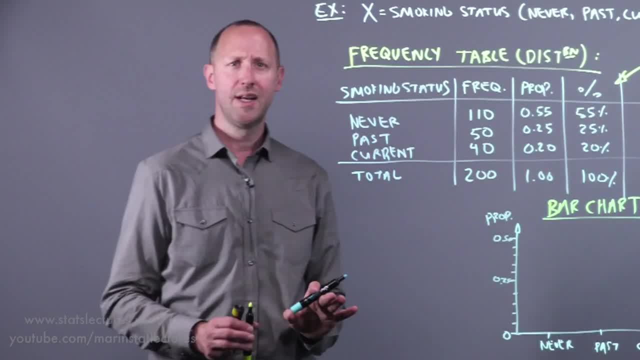 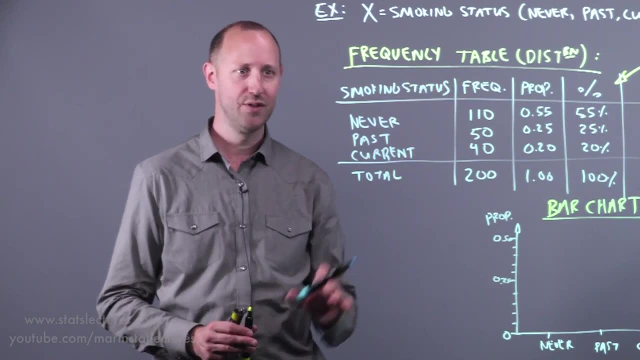 Up here: .50, .25.. And it's important to mention here: you probably will never create any of these by hand, right? Use a computer or a piece of software to do these. We're going through and looking at doing them by hand. 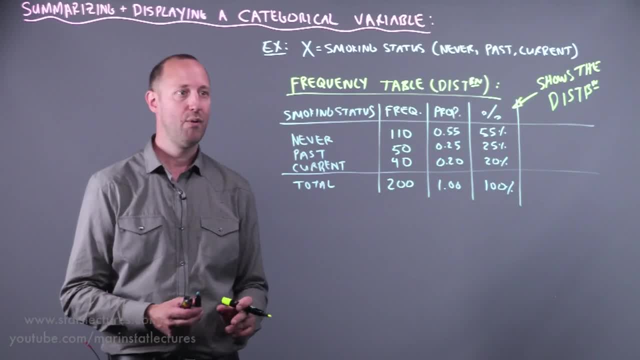 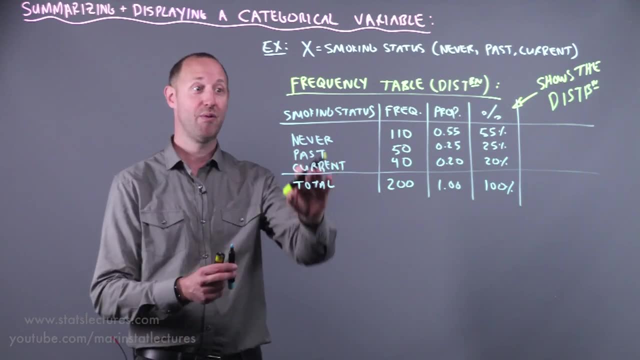 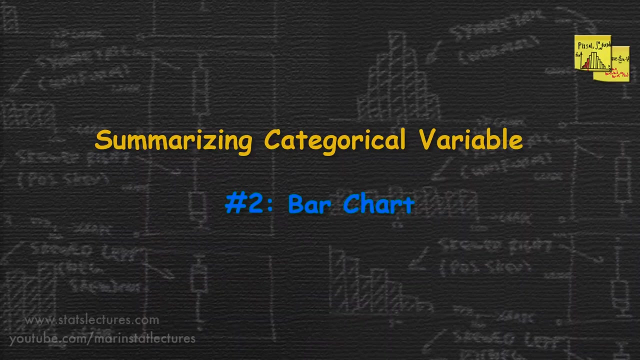 be a bit misleading with smaller sample sizes. now, if we want to make a plot of these right, it's nice if we can make a visual of this table rather than just looking at a table of numbers. especially when the table gets bigger, we can make either a bar chart or a pie chart. so first let's start by 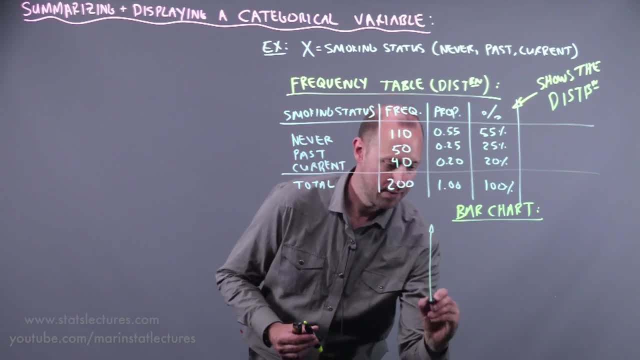 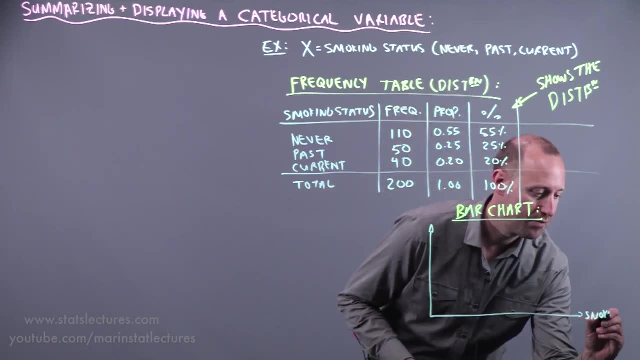 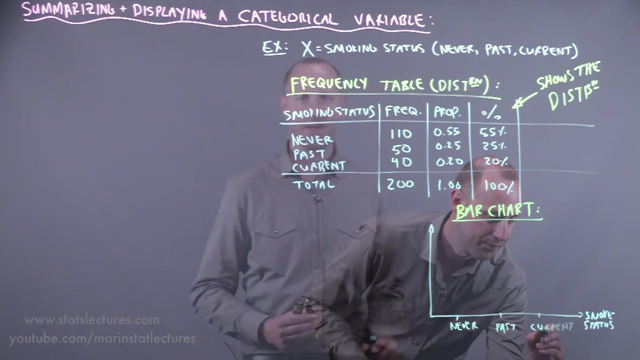 talking about the bar chart. a bar chart has along the x-axis the variable. so here we're looking at smoking status again. this was recorded as never past or current, and along the y-axis we can put the frequency, the proportion or the percentage. right, the plot's going. 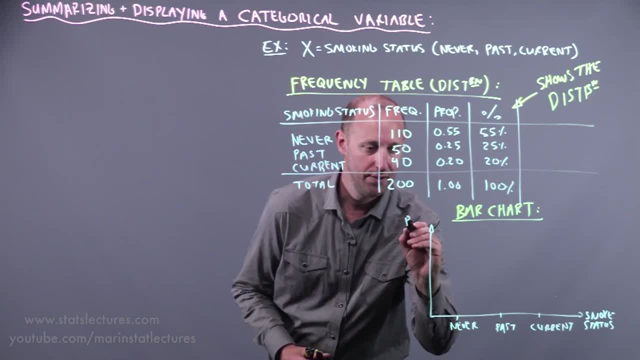 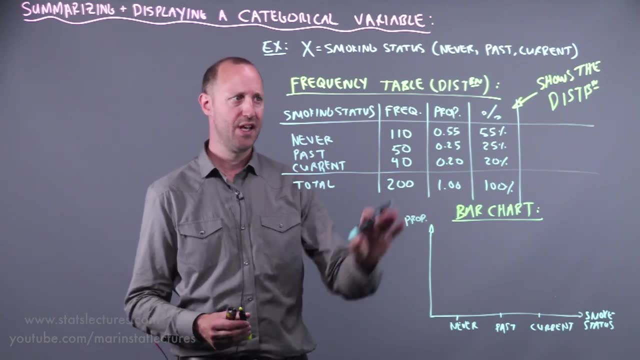 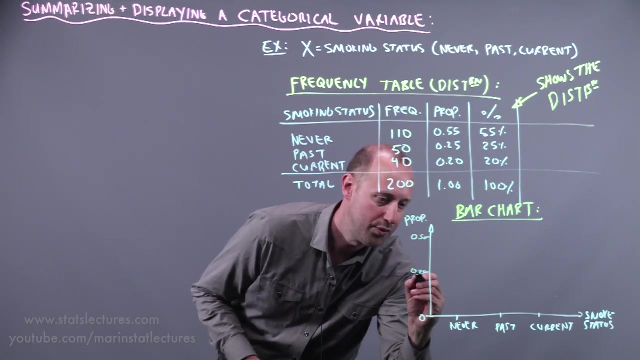 to look the same, i'm going to choose to put the proportion here, since our sample size is not very small. i think it's more meaningful to report proportions or percentages and i'll just choose the proportion down here. we'll put 0 up here, 0.50, 0.25, and it's important to mention here. 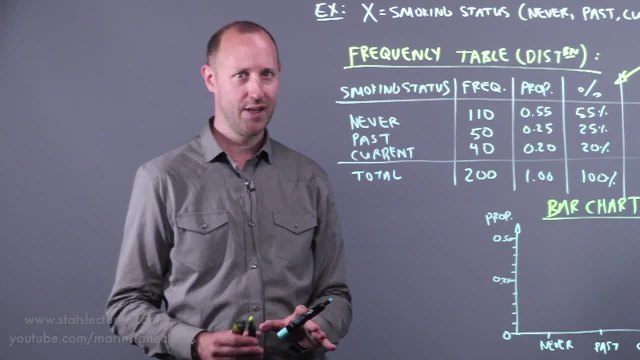 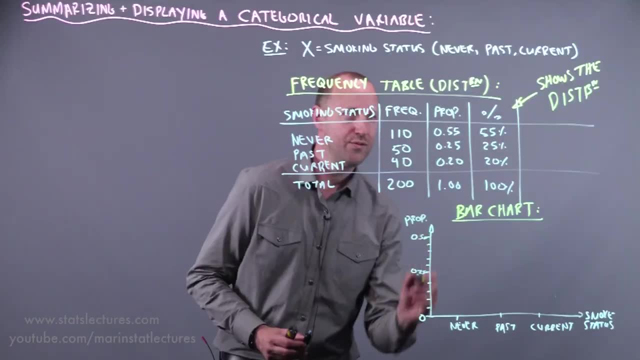 you probably will never create any of these by hand, right, use a computer or a piece of software to do these. we're going through and looking at doing them by hand for the sake of discussing the concepts and what they are. for the never smokers, they have a proportion of 0.55, so roughly up here. 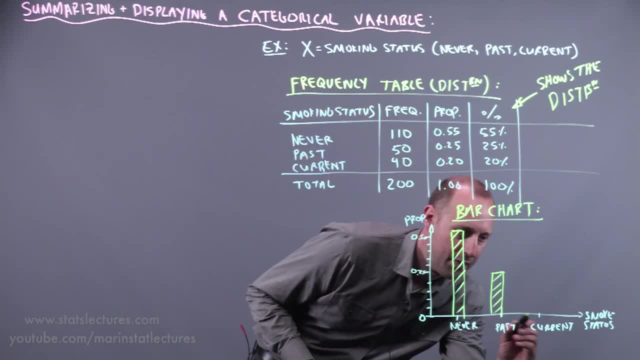 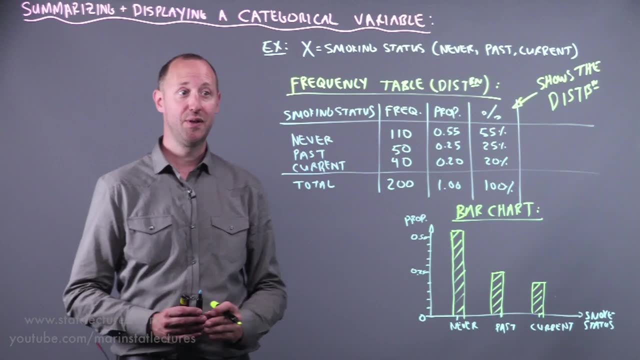 for the past smokers a proportion of 0.25 and the current smokers a proportion of 0.20. now, in this plot, these bars are separated or spaced between them, again to indicate that these are separate categories. there's no continuity between the two and as though to be a bar chart. it's not going to be a bar chart, it's going to be a bar chart. 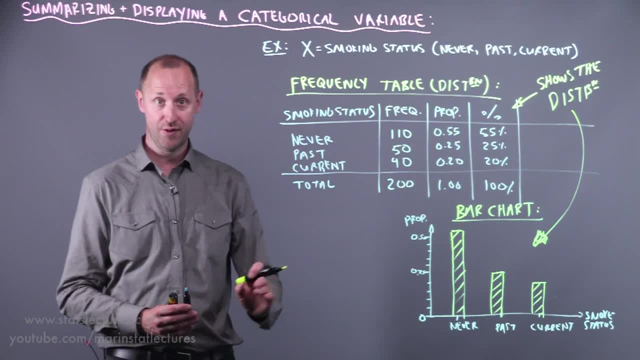 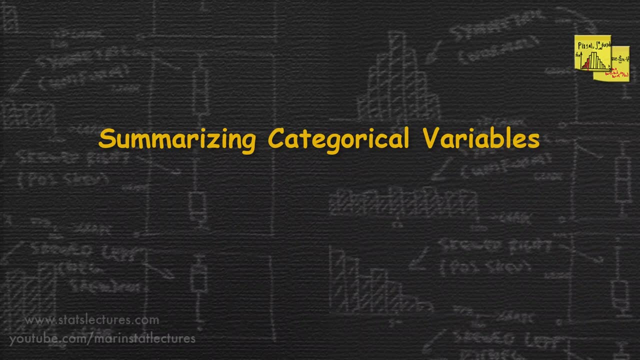 this here also helps show the distribution for this variable right. how are people distributed amongst the different categories or levels? the one other plot that we can make for this table or for a categorical variable is a pie chart. the way a pie chart works is you start with a. 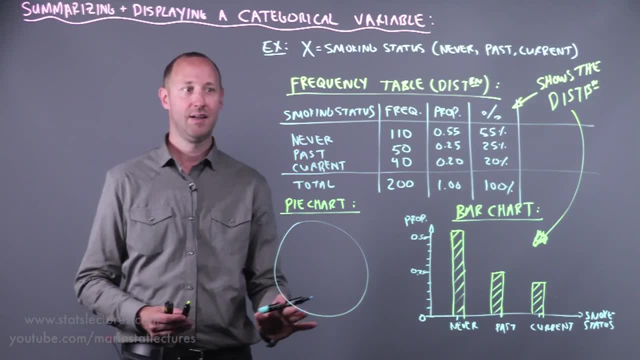 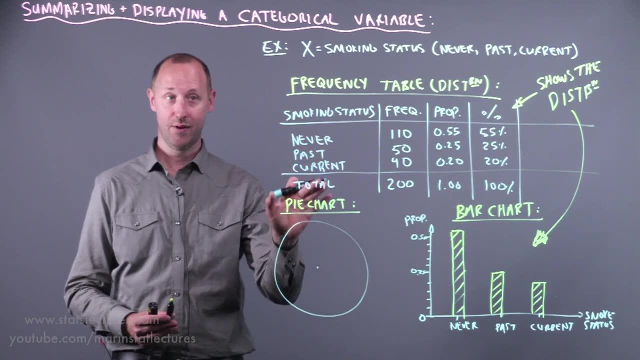 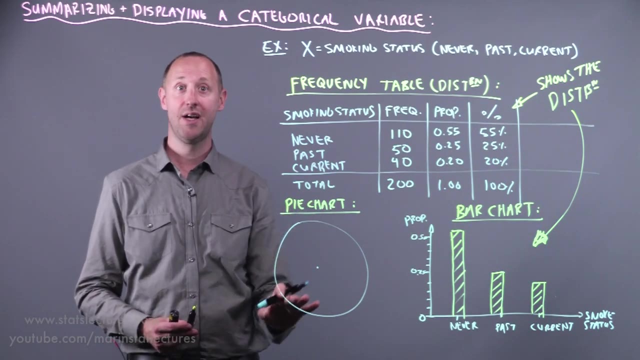 pie, right, or a circle, and again this pie or this circle represents the entire sample. then what we do is, for each category- right, or each level or category of this variable, we draw a slice of the pie, and the slice of the pie should be proportional to the percentage of the sample they represent. so let's start with the past smokers. 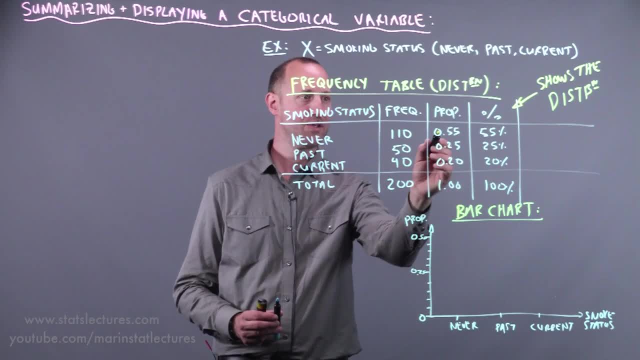 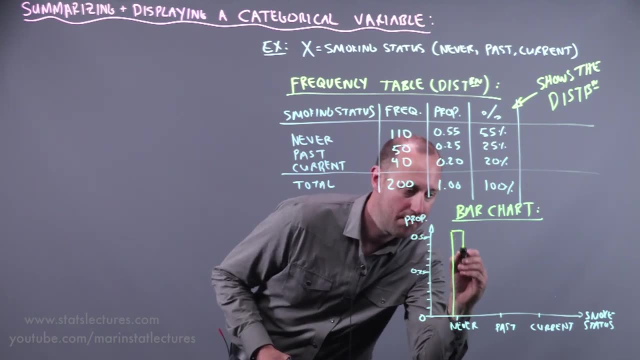 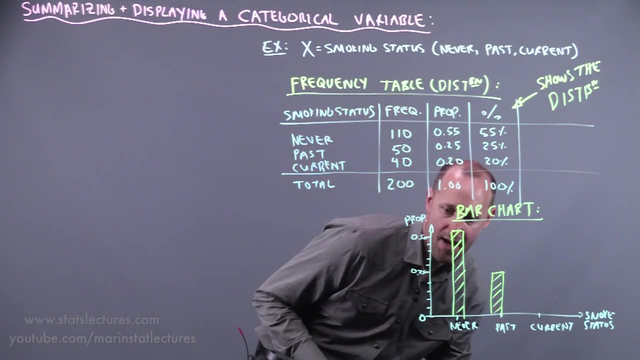 for the sake of discussing the concepts and what they are. For the never smokers, they have a proportion of 0.55.. So roughly up here, For the past smokers, a proportion of .25.. And the current smokers a proportion of .20.. 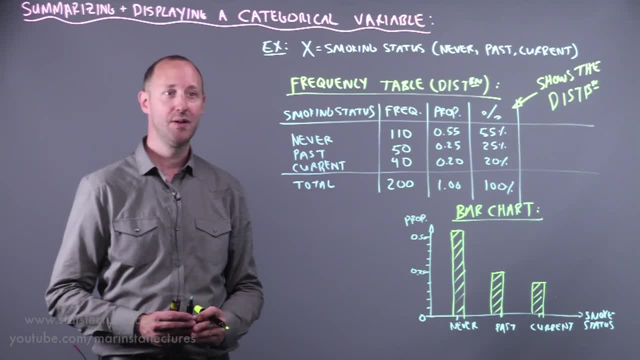 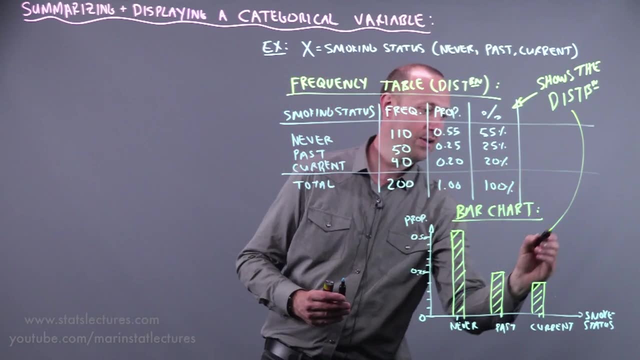 Now in this plot, these bars are separated or spaced between them, again to indicate that these are separate categories. There's no continuity between the two And, as noted before, this here also helps show the distribution for this variable right. 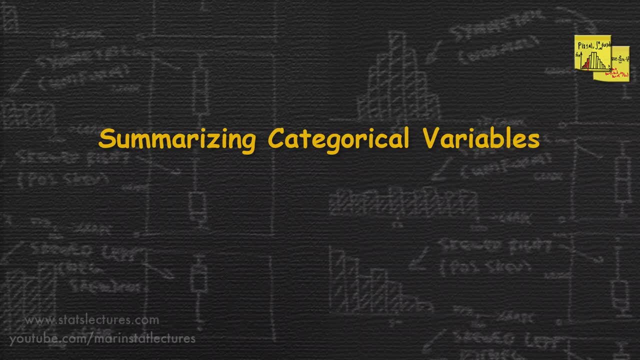 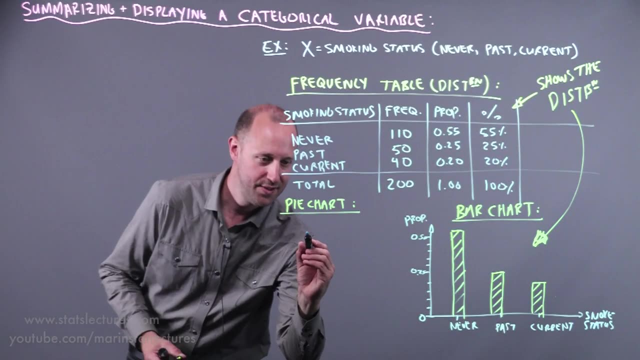 How are people distributed amongst the different categories or levels? The one other plot that we can make for this table or for a categorical variable is a pie chart. The way a pie chart works is you start with a pie right Or a circle. 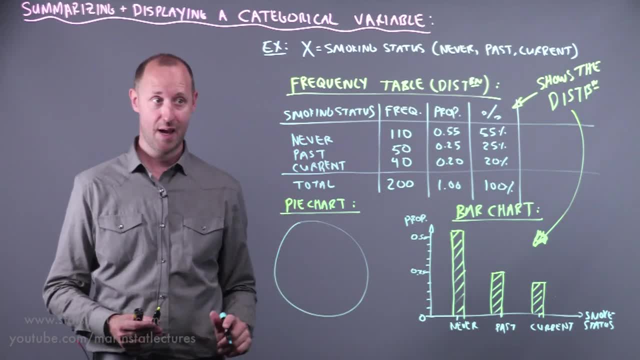 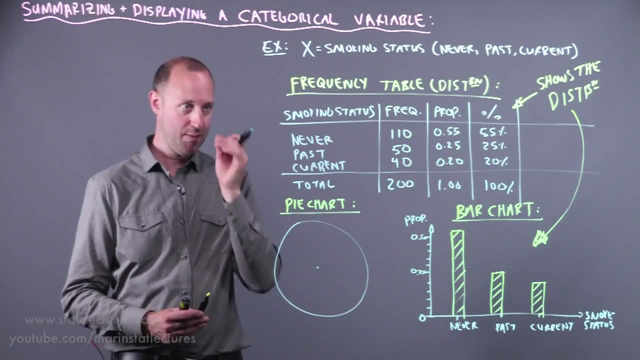 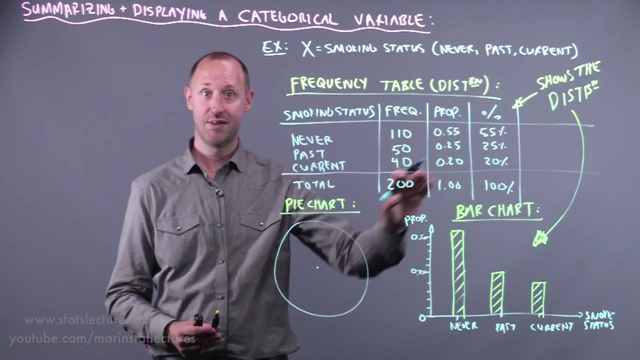 And again, this pie or this circle represents the entire sample. Then what we do is, for each category, right For each level or category of this variable, we draw a slice of the pie, And the slice of the pie should be proportional to the percentage of the sample they represent. 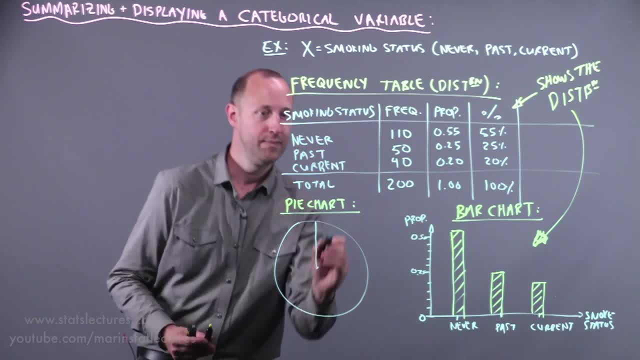 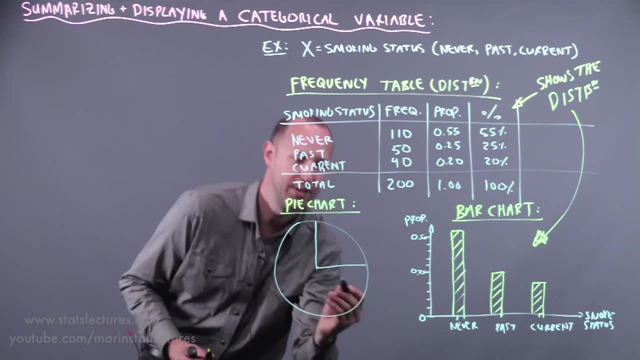 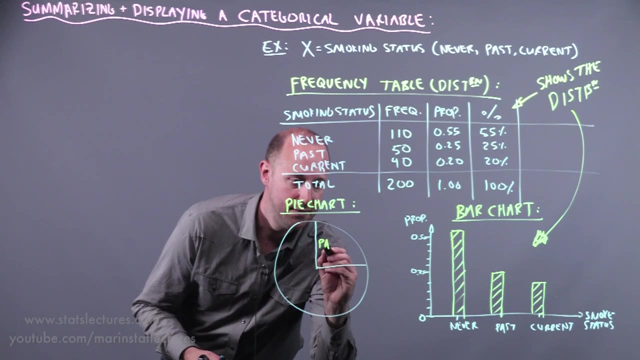 So let's start with the past smokers. They're a proportion of .25 or 25% of our sample, So I'm starting with that because that's the easiest one to draw right. It's one quarter of the pie, And I'll label this here as being past. 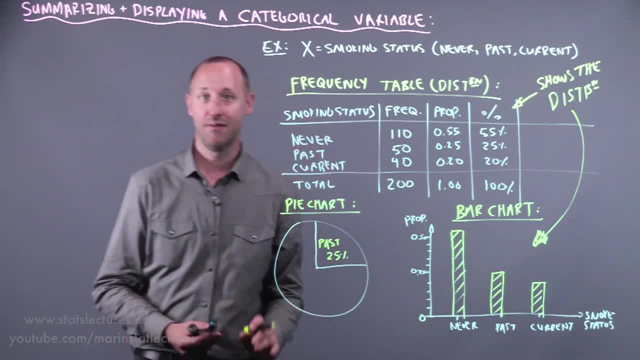 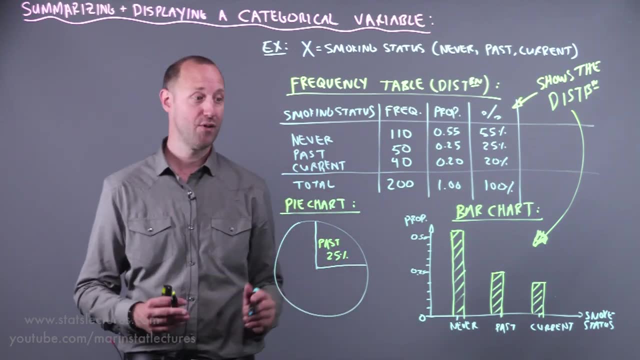 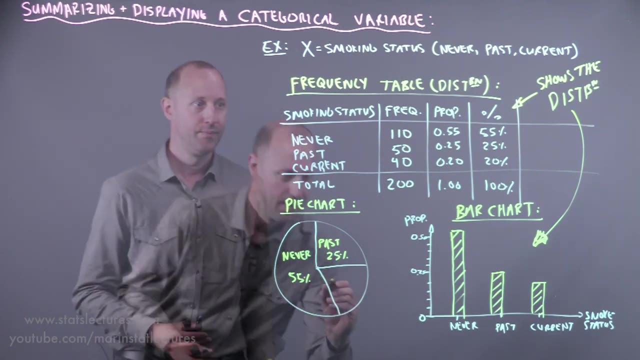 These are the past smokers, And it's also nice if the percentages or proportions are written in there. The next are the never smokers. They represented .55 or 55% roughly here. These are the never smokers- Again, 55%, And the current are 20%. 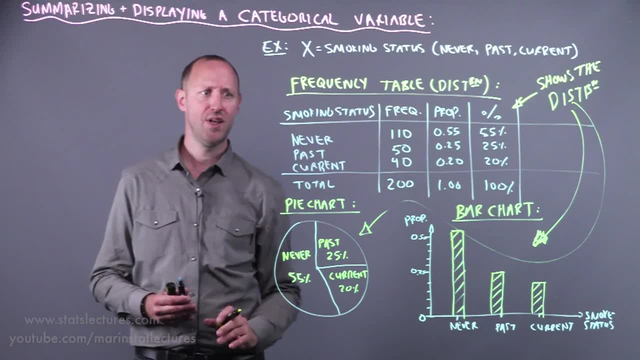 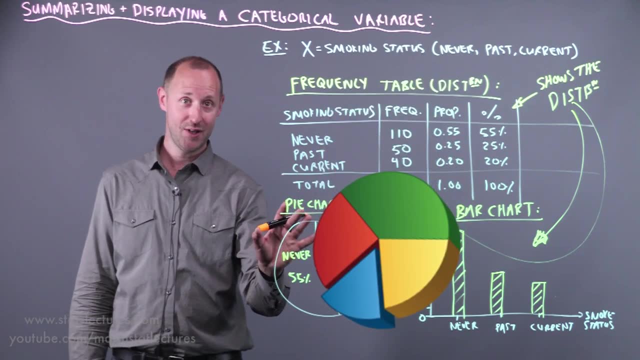 This here shows the distribution for our sample. So another visual way of showing this. So one personal preference I want to mention here. while you often see these 3D pie charts shown because they look kind of cool, I'm going to really recommend that you don't do those. 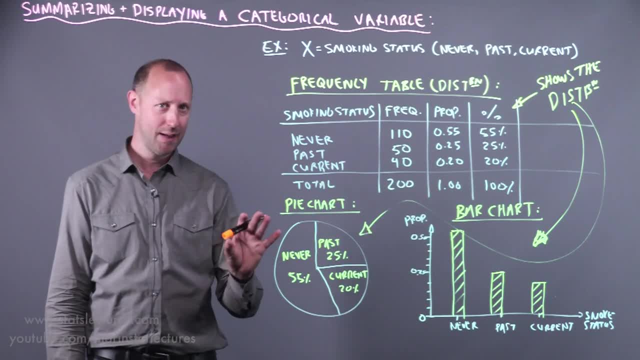 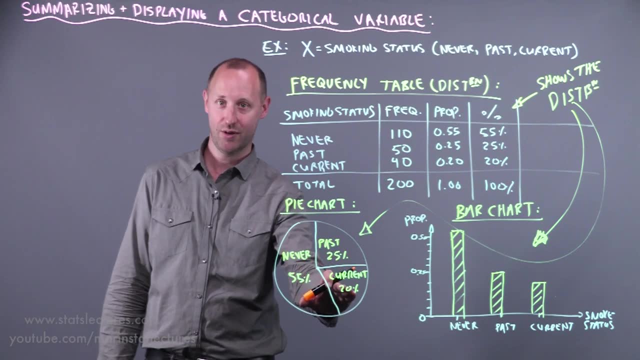 And it's because they violate one of the main principles of producing a plot, And I'm going to show you that here And well, my drawing's not perfect here, but the slice for the past smokers should be a little bit larger than the current smokers.